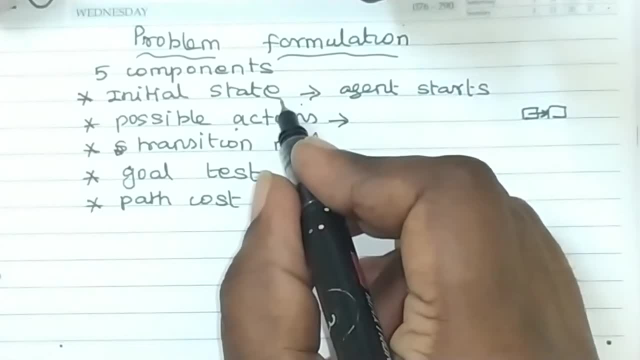 So and the actions? What are the actions? from the other, The possible actions, What are all the actions can be performed by that particular problem solving agent is called as actions. So next, the third one is transition mode. So, the third one is transition mode. 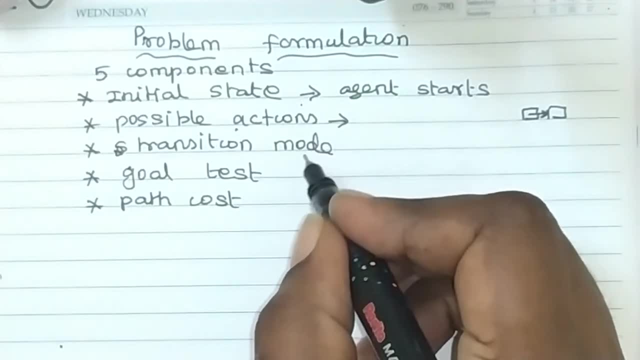 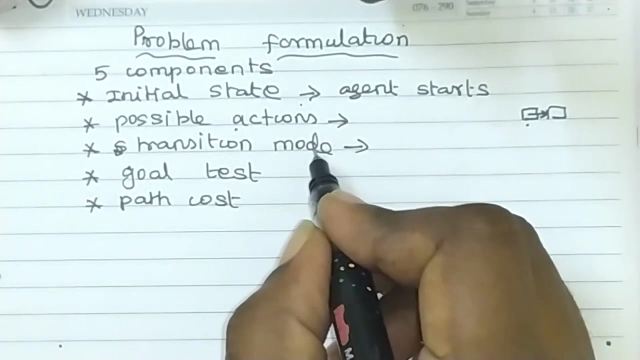 The transition mode is nothing but the action is which we just learnt it. The action has a lot of actions. When the only actions moves, then the agent moves from one state to another state. The moving state means the transition mode. The fourth one is: 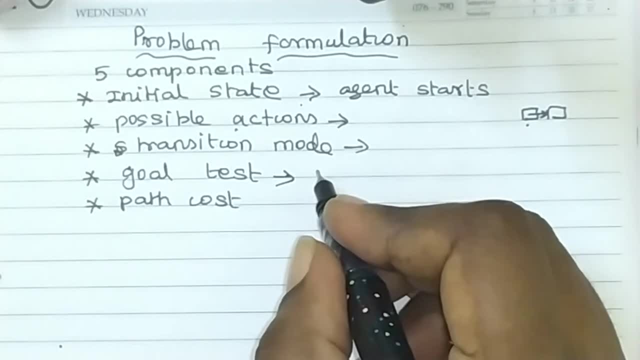 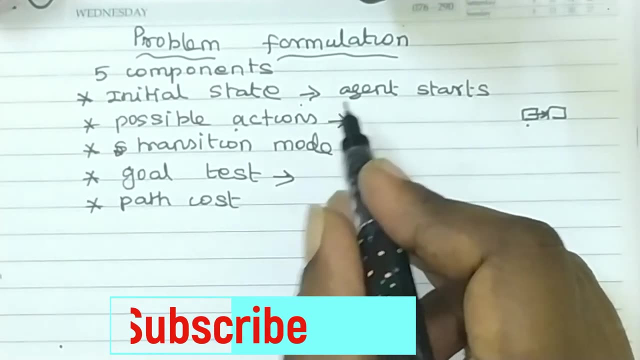 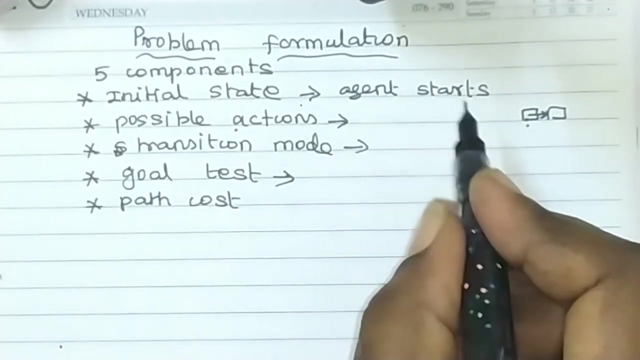 goal test. So this goal test determines whether a given state is a goal state. So so if all the origin with the action of performance, performance, so the state is changed from one state to another state, so far I know the state change of mother and the particular state, the world's state, are eventually check. 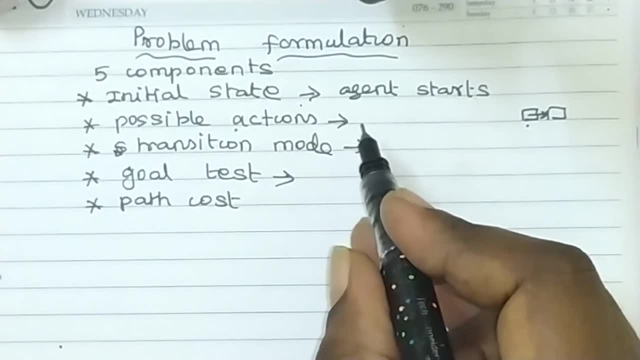 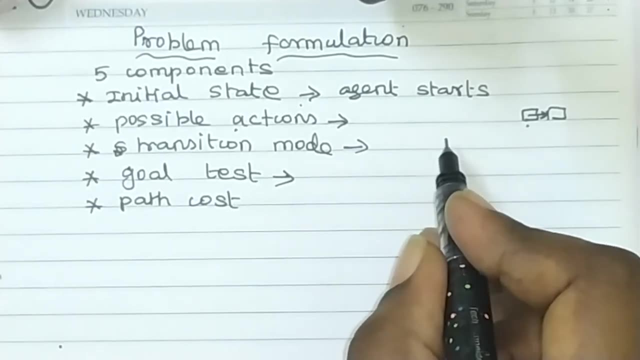 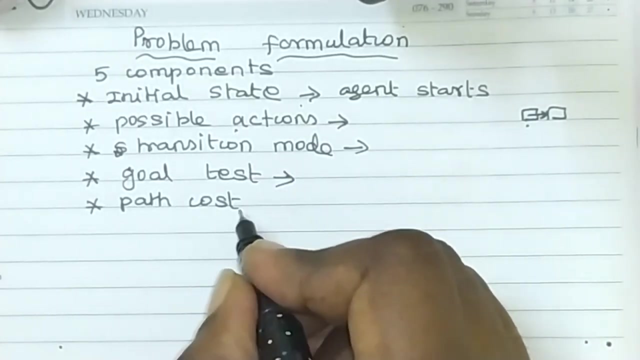 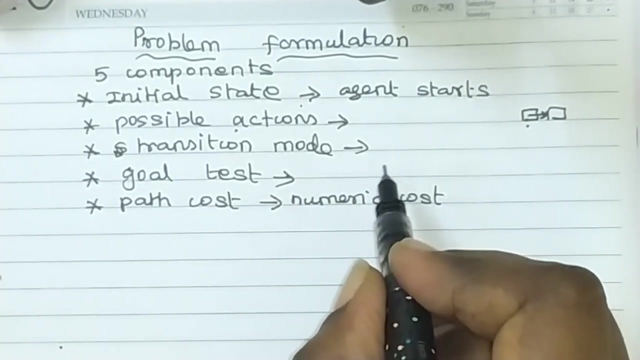 the gold, just the state change of the. we have to check whether the particular state is a whole state armor. that can be done by the school just next. last component is podcast, podcast, Nana. so it assigns a numeric cost, unique cost of each path for a father. so it will state on a mom why you finally will go and I'm a reach. 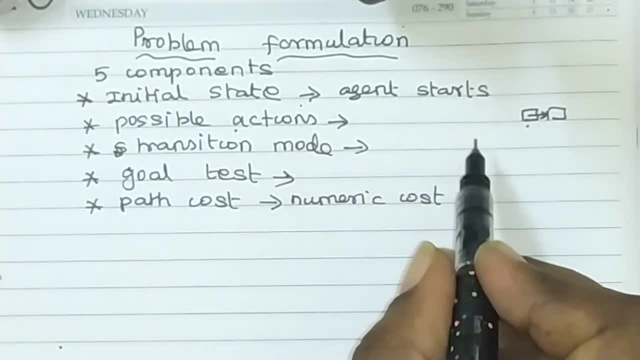 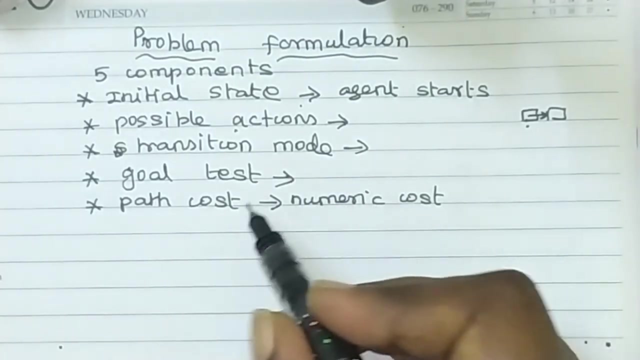 point in a real states of the moment, when me and the whole- and I'm a reach point of support for state to go, we have to assign some memory cost, so that cost is called as podcast. so finally assigns a memory cost to each path of a podcast. 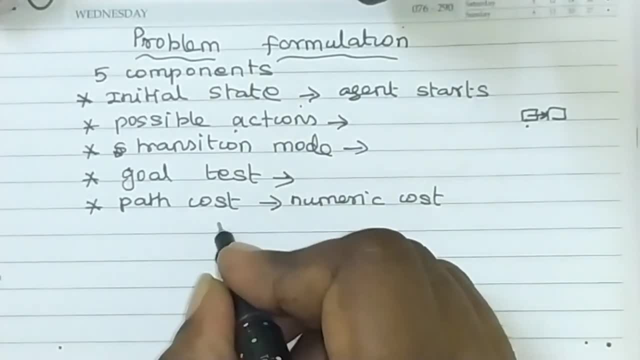 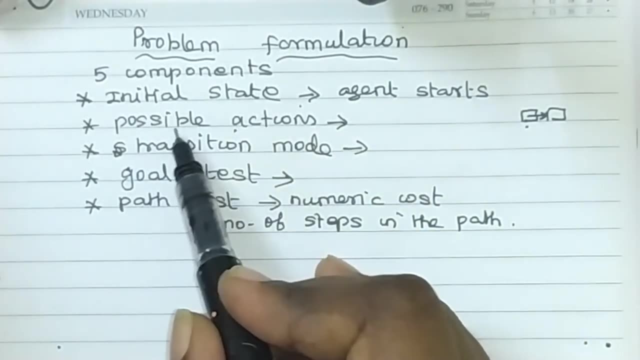 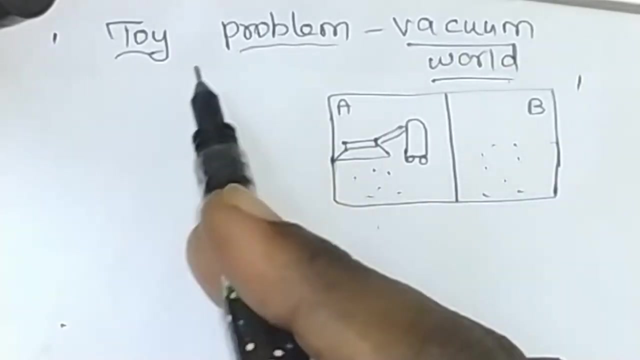 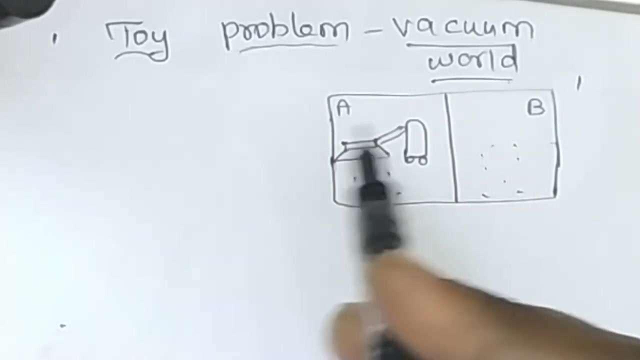 Nana, a partition stage, transition or gold test and webcast problemle problem wherever, like a gold problem, when the possible on in the problem like capчно the problem. the formula on historyочку 요즘 is, I think, the concert a problem solving page. 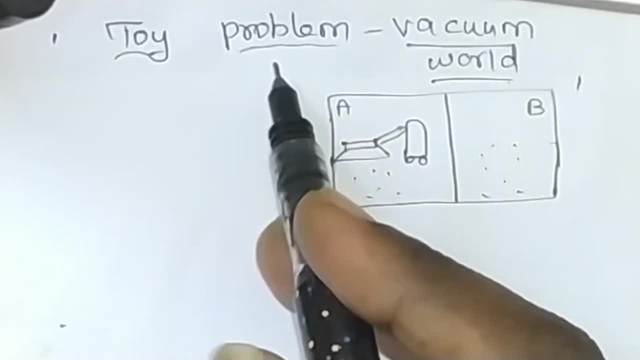 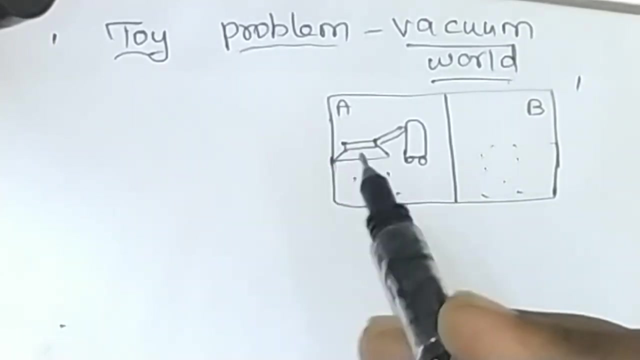 problem-solving agent is to formulate the problem using five components: initial state actions, transition mode, goal test, path cast. we have already seen in the previous video, so in this video we are going to see how the problem-solving agent formulates the toy problem. 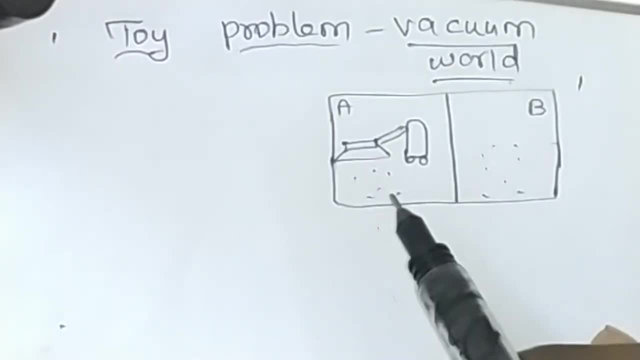 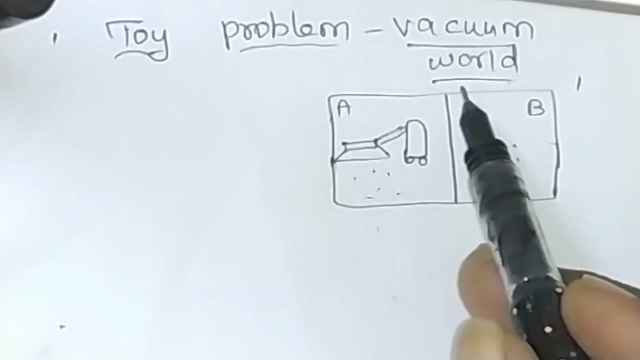 there are two squares, A square and B square. so vacuum cleaner is placed in any one of the square, A square or B square. vacuum cleaner is placed in any one of the square, so if A square contains some dirt, then the vacuum cleaner will clean that dust or dirt. 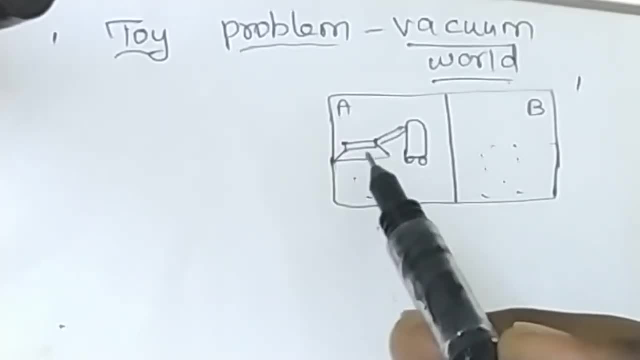 so now, vacuum cleaner, after cleaning the dirt in A square, what will it do? it has to move to the next square. move to the next square and check if the dirt is in that square. if there is any dirt is present in that square. there also, it has to perform some action. 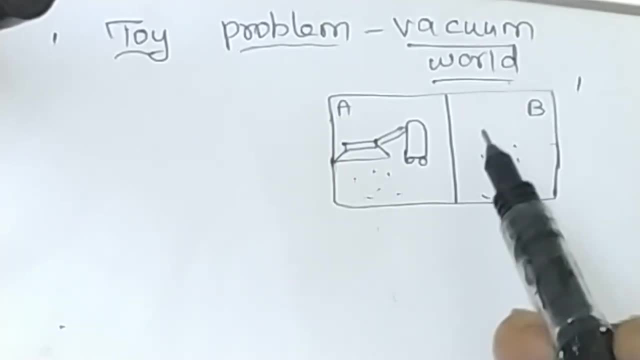 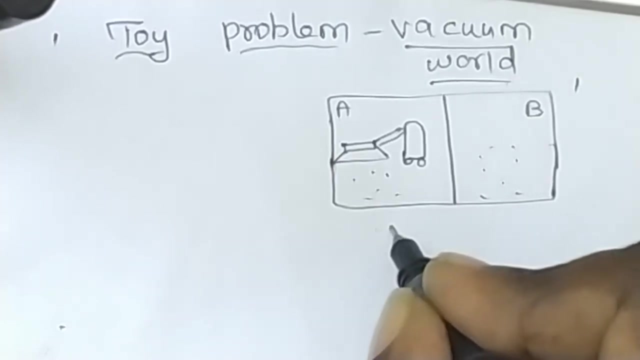 so once the action is performed, the state is changed from one state to another state, one state to another state. so in this kind of problem we have to find out how many states are there. in this problem there is a formula, so 2 into 2 power n. 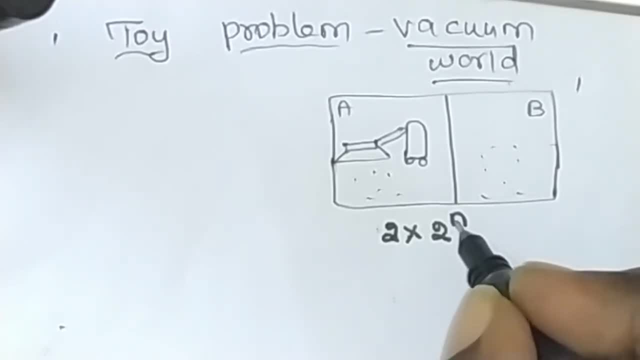 n is called as locations. here n is called as locations, so in this problem we have taken only two locations, so n becomes 2. now 2 into 2 power 2. so totally for this problem we can get 8 possible states in the world. what are the actions that an agent can perform? 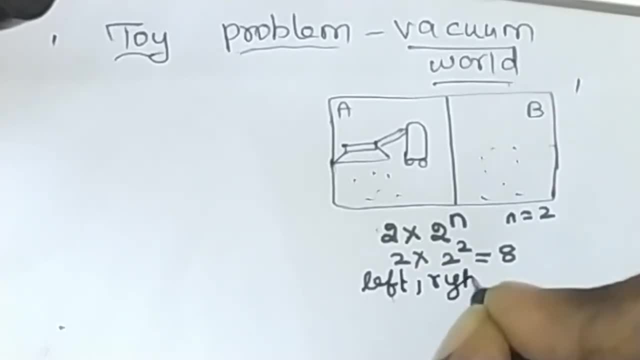 left, right, suck and do nothing. so if any action is not performed, that is why I can do nothing- so we can use this, which means we can do either right or right action. we can do suck action and we can clean the dirt, and this is the suck operation. 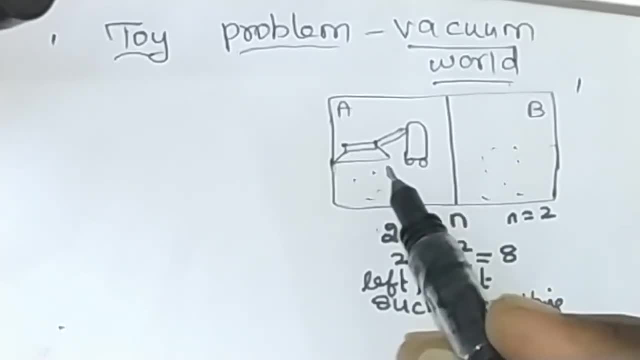 why the square is clean like this. the vacuum cleaner does the following: it has to perform one action. that action is called as move right, so the vacuum cleaner immediately moves to right. it moves. now. let's suppose there is dirt in b dirt and the suck. it will perform the action: suck, suck, action. 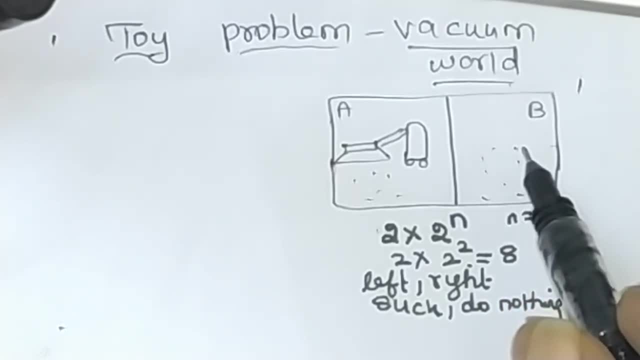 moolama dirt and clean it. so if the b-square is clean, so next it has to move to the s1, so both of the squares are clean, so the problem is solved. so this is called as back of world problem. so now we are going to formulate: 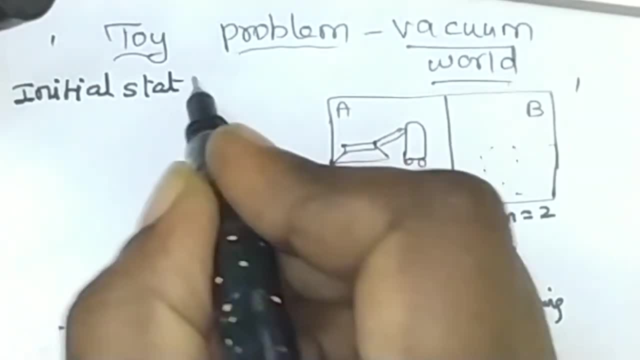 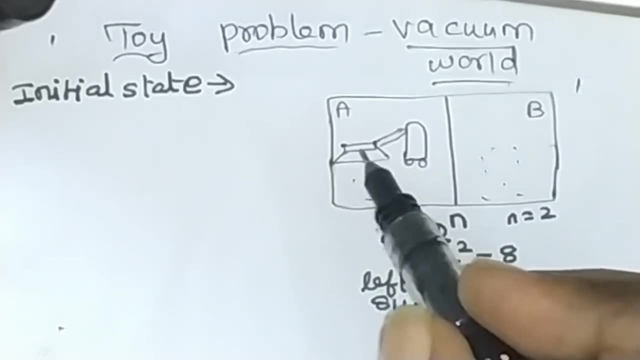 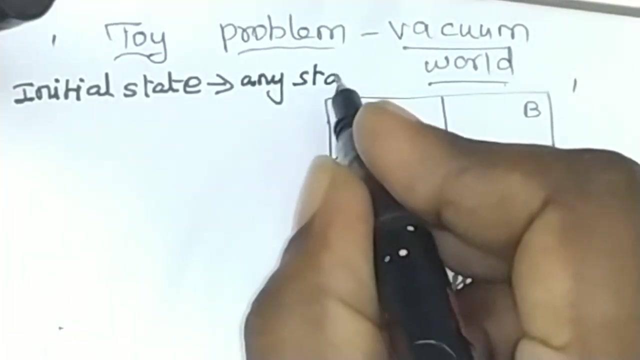 state. so in the problem, initial state. now any state is designated as the initial state. so by comparing, if a is suppose, a is place, that is the initial state. if b is place, that is the initial state. so that is the first one, any state. next is actions. so what are actions? 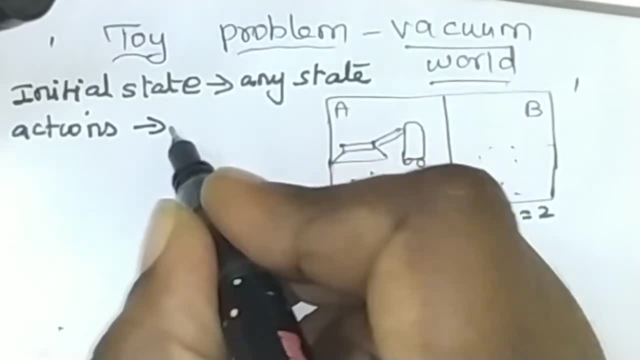 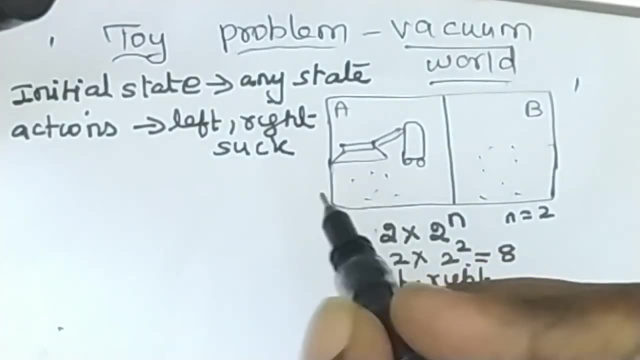 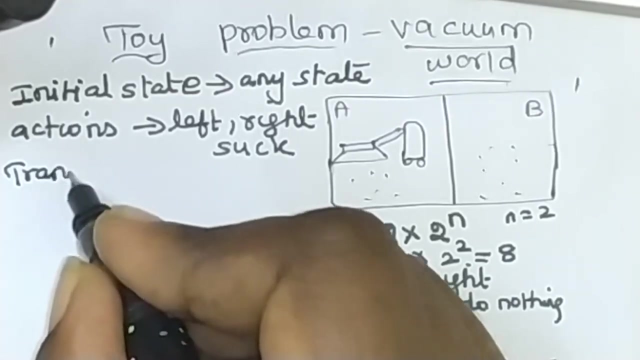 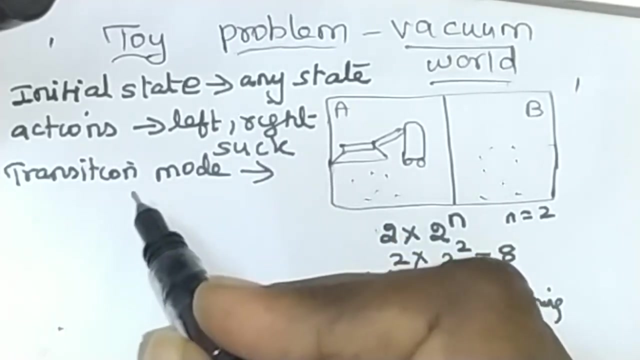 a complainant: 100. so in an action, let it to the main. actions are left to right. so these three actions performed by thispetas. next one, the transition mode. the state is changed from one state to another state. so actions have expected effects: actions for the effective actions. a performer move state when the change of 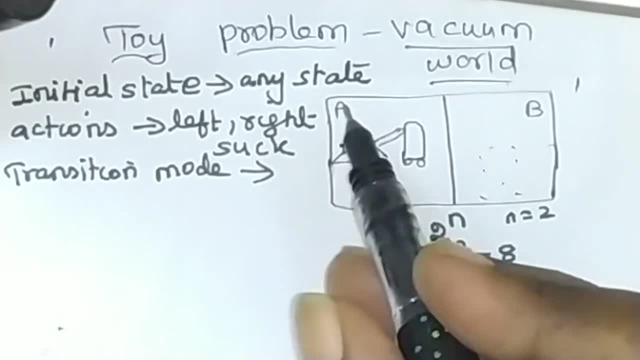 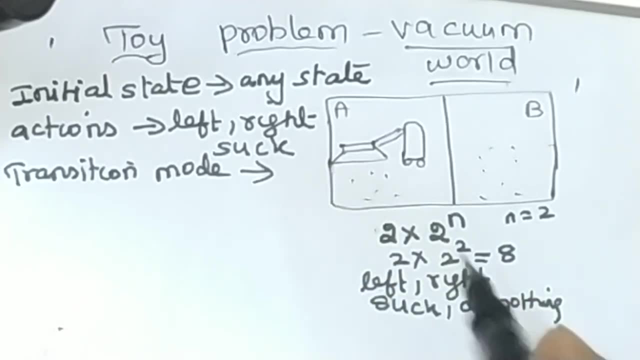 that is called as transition. if suppose angry location of the dirt on so in action weapon be my performance suck. so once this suck operation is performed, suck action is performed, the state is changed, that is, a square is declared as the clean square. so clean I jump into the moment in the car. so initial action: